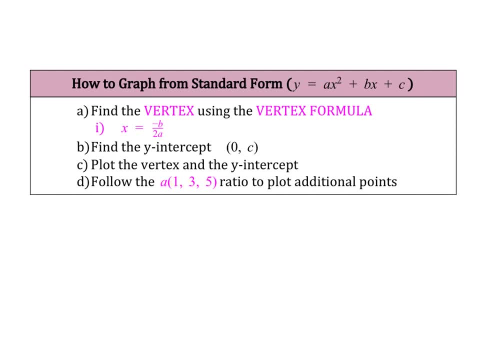 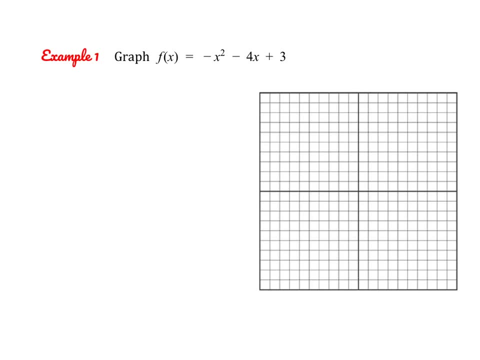 We multiply this ratio by your, a value to adjust for that vertical stretch or shrink. So let's go through one together. So remember, step one is always to find the vertex And of course, to do this we're going to use our vertex. formula x equals negative b over 2 times a. 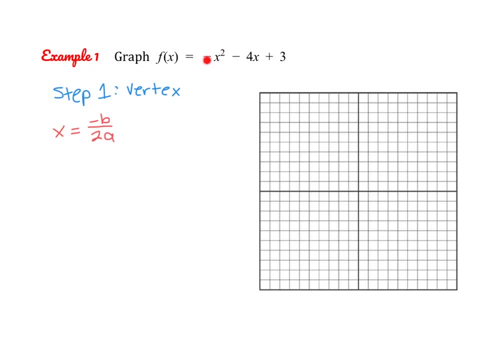 And then I look at the formula, I look at my equation and I can see that the coefficient of x squared is negative 1.. So I'm going to say a equals negative 1.. And then I need to find b as well. 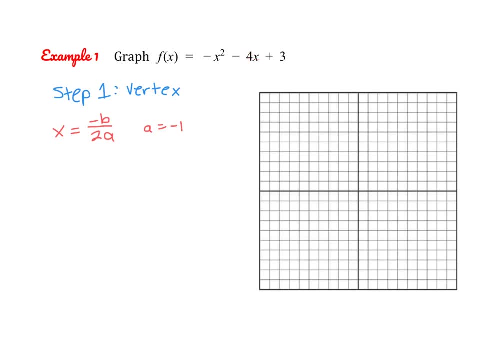 So I look at the coefficient of x and I see negative 4.. So b is negative 4.. So let's do our substitution: x equals negative, and then I always substitute with parentheses: b is negative 4,. so notice, I have two negatives. 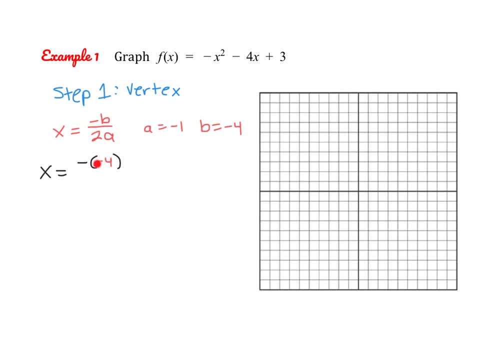 This negative is from the formula, this negative is from my b value. And then I do divided by 2 times, and we're going to substitute a with negative 1.. And now we simplify Negative times: negative 4 is positive 4.. 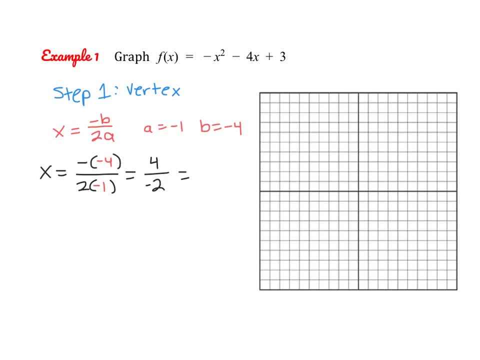 2 times negative, 1 is negative 2.. So we get x equals negative 2.. So now I need to find the y value of our vertex. So again, this is just the x value of our vertex. To find the y value we do f of negative 2.. 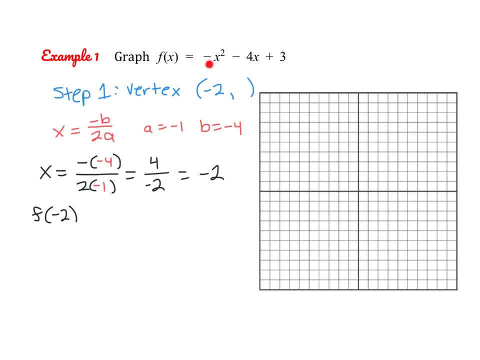 So now I'm going to take my x value and I'm going to substitute it into our equation. So negative 2 squared minus 4 times negative 2 plus 3.. Notice, when I do this, the negative is still there, The squared is still there. 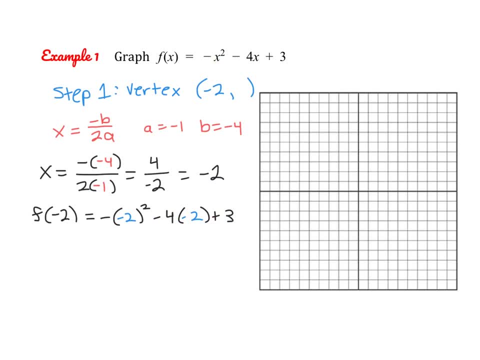 Negative 4 is still here, plus 3 is still here. I'm just replacing any x with negative 2.. So now I'm going to start following my order of operations. to simplify, We always start with our exponent, So we have negative. 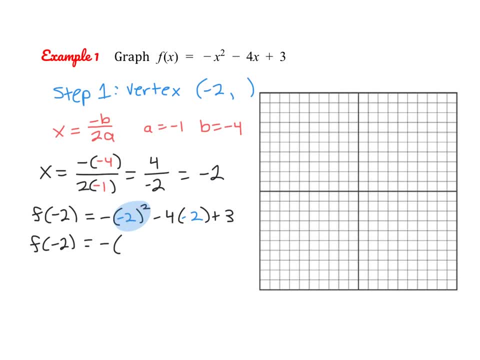 Negative 2 times negative, 2 is positive 4.. Minus 4 times negative, 2 plus 3.. And now we can do our multiplication Here and here: F of negative 2 equals negative 4 plus 8 plus 3.. 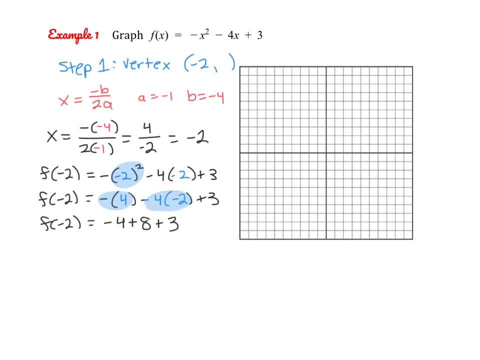 Because, again here, negative 4 times negative, 2 is positive 8. And now we're just going to simplify by adding or subtracting. So negative 4 plus 8 is 4 plus 3 is 7.. So our vertex: 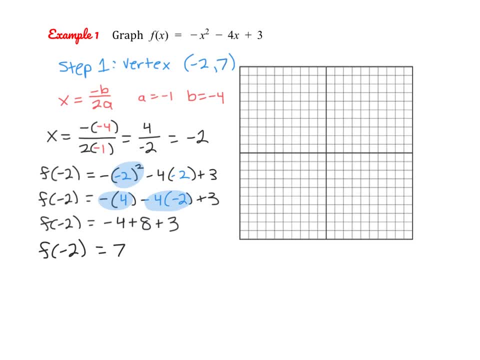 Our vertex is at negative 2, 7.. So when x is negative 2,, y is 7.. Okay, so now we can move on to step 2. Which is to find the y-intercept. So remember, our y-intercept is always going to be 0.. 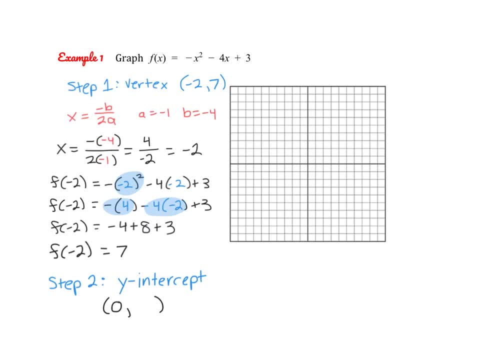 And then our c value. So if you look back up to our, To our original equation, our c value, which is always the constant, And again the constant is the number, without a variable. So I can see that my c value is 3.. 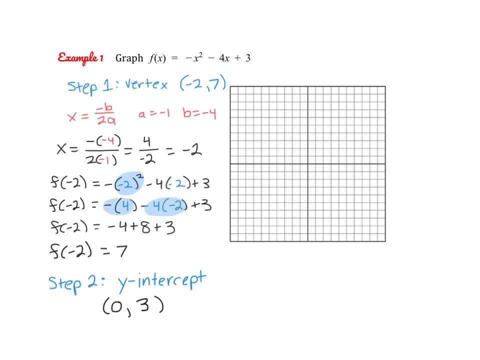 So I'm going to place 3 as my y-intercept. So now I know my vertex and my y-intercept, So we can move on to step 3, which is to plot those points. So my vertex is negative. 2, 7.. 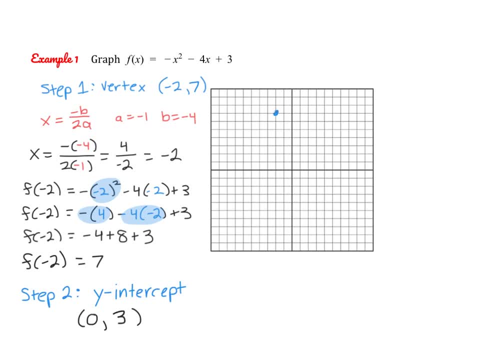 So it goes right here And my y-intercept is 0, 3.. And now I have to figure out a few additional points in the graph And I am going to make my parabola. So first thing I notice is that my a value again is negative 1.. 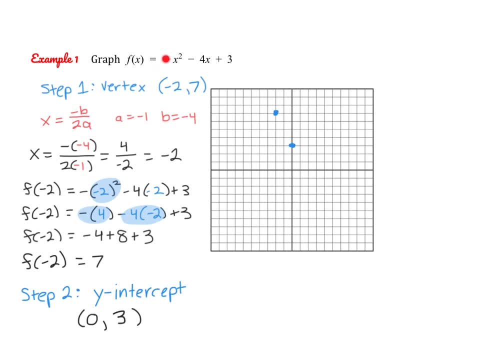 I want to remind you guys that when our lead coefficient is negative, we have a negative graph. It looks like a sad, It's a sad face. It's a downward-facing parabola To find more exact points. I want to remind you guys that we do our a value. 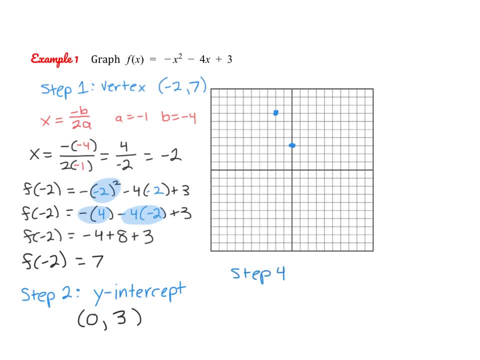 So this again is: This is now step 4.. We do our a value, which in this case is negative 1, times our 1, 3, 5 ratio, And that tells you where to go for the next points. 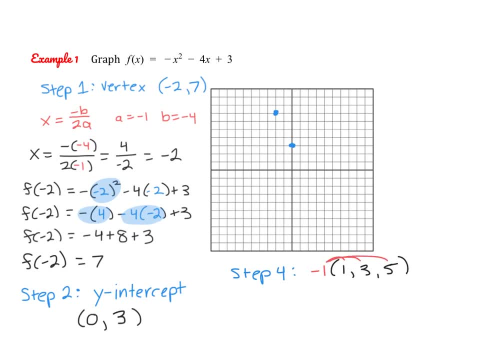 So, instead of negative, Instead of 1,, 3,, 5, we distribute And the ratio is negative: 1,, 3,, 5.. And the ratio becomes negative: 1, negative, 3, negative, 5.. So this tells us to start at the vertex. 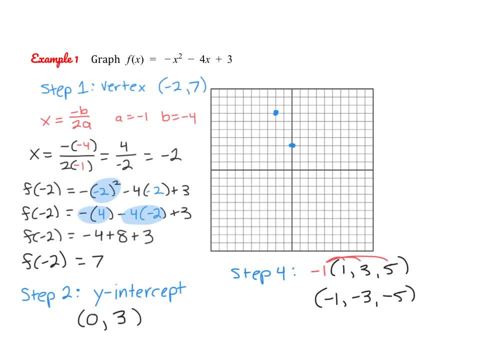 And I go down 1 over 1. And that's where I put my coordinate. And then I go down 3 over 1. And that's where my next coordinate would be, which I already have one there, which is good. 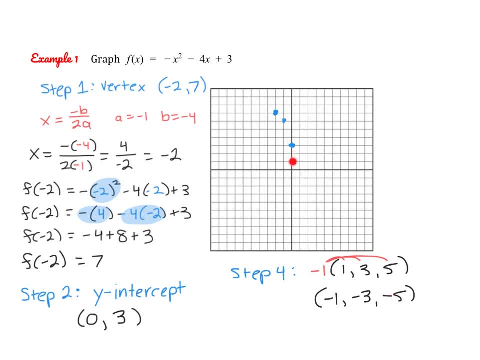 And then I go down 5 over 1.. 1,, 2,, 3,, 4,, 5 over 1.. So remember, this tells you This ratio, tells you how to get to the next point. So I go down 1 over 1, down 3 over 1, and down 5 over 1.. 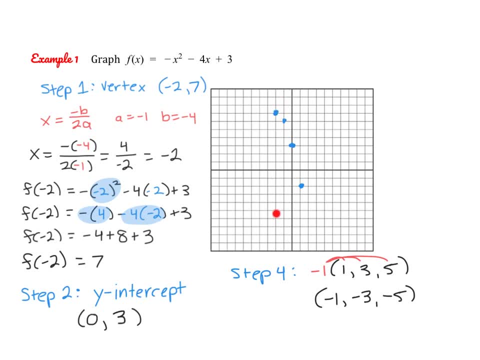 And now I know that, since my axis of symmetry is always right through my vertex, I know that all of these points are going to be reflected onto the other side. So just to kind of show you guys, Here's my axis of symmetry, So now I can reflect those points. 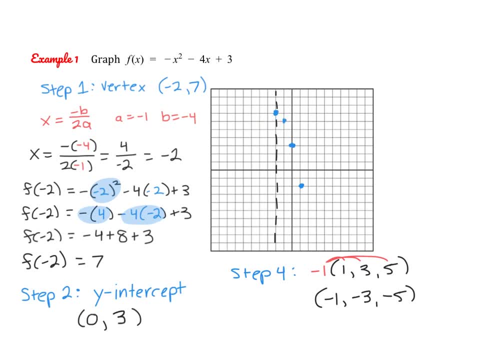 This coordinate is one unit away, so I'm going to go one unit away. on the other side, This coordinate is two units away, so I go two units away on this side and I put my next coordinate And this coordinate is three units away, so I go three units away here. 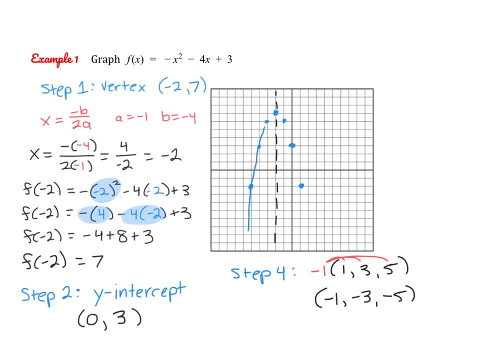 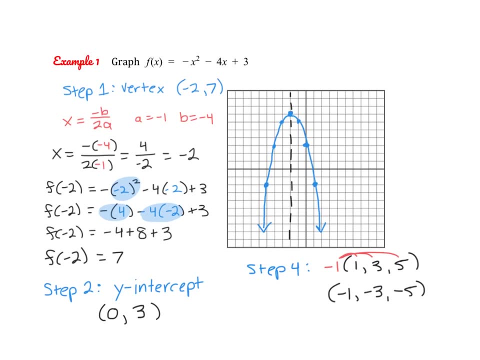 And now, if you connect your dots, you'll see that we have a downward-facing parabola. Okay, And this is going to be the next parabola. So there you go. So again, the process- because you're about to try one on your own- is to find the vertex. 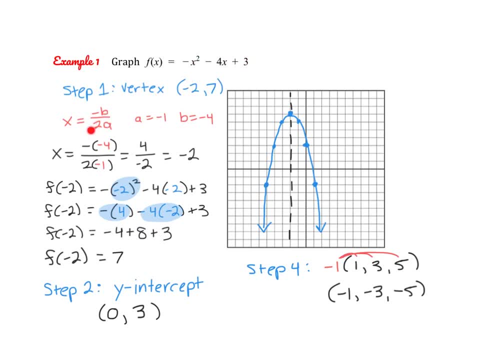 Now, when it's in standard form, we have to use our vertex formula. so we have to use x equals negative b over 2a. So you find your vertex and then you find your y-intercept, which is always going to.